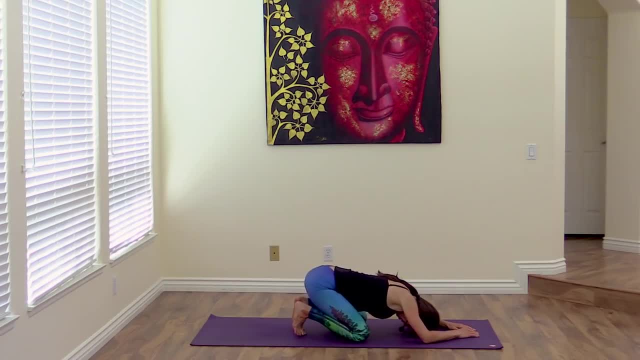 Rest your forehead down on the ground-ish Arms in front of you, elbows softly bent, And in yoga, the entire practice is built around the breath, And so what we practice with yoga is mindful breathing As well, as we smooth the breathing out and slow the breath down. 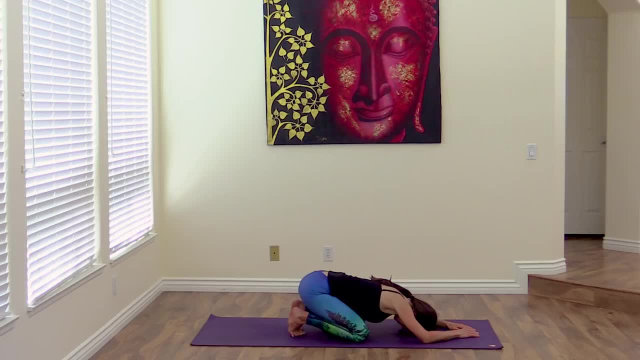 So begin to breathe through your nose And smooth out your breath. So if somebody were to listen to you breathing right now, they would naturally assume that you were in a calm mindset. All right, so the breath isn't choppy or erratic. 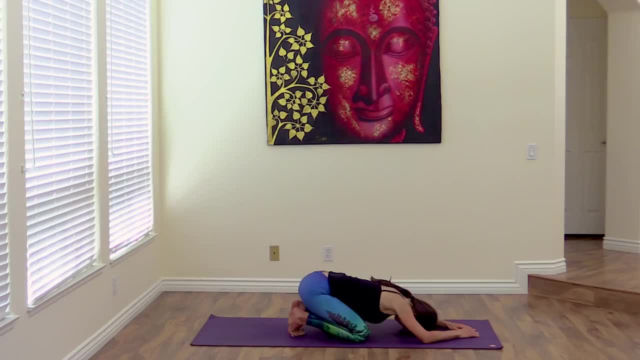 It's smooth and deep, Good. and then you'll come up to your hands and your knees- Hands under the shoulders, Knees up Under the hips. We'll move through some cats and cows. Maybe you've done these before On an inhale. drop your belly down. 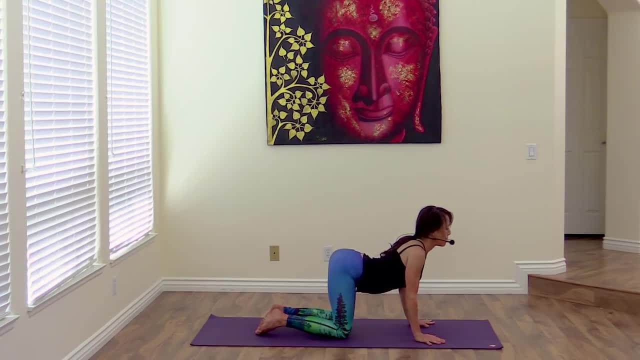 And arch your back to a back bend And then, as you exhale, round in through your spine, Tuck your chin into your chest On an inhale, drop the belly down, Pull the heart forward, Arch your back As you exhale. 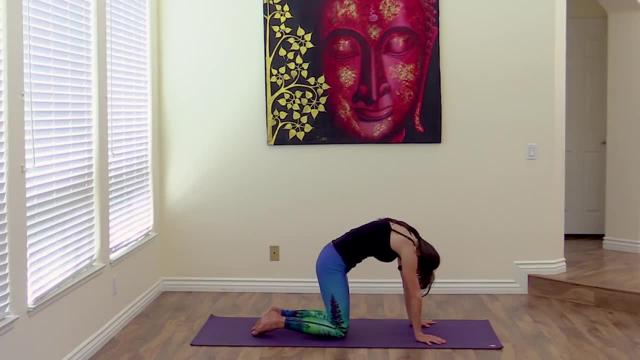 round through the spine, Tuck the chin in and feel a nice stretch in the upper back, Maybe the lower back too. A few more times, Linking the breath with the movement: Inhale, Arch your back, Exhale. 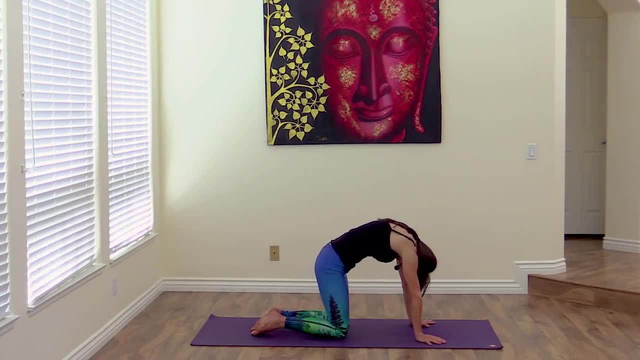 Round in through your spine One more time. Inhale, Arch your back, Exhale, Exhale, Round in Beautiful. Now come to a neutral spine, a flat back, And we're going to come into downward facing. dog pose is what it's called. 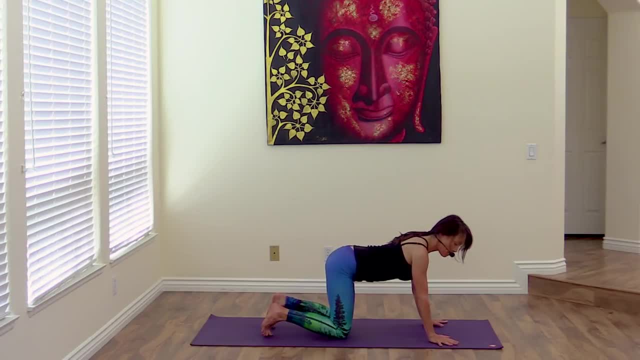 The hands can turn out just slightly, And do be mindful that the wrists they're either straight, like aligned with the front edge of your mat, or turned out a little bit. The fingers are spread and the hands are not too close together. So you want the hands at least shoulders width apart. 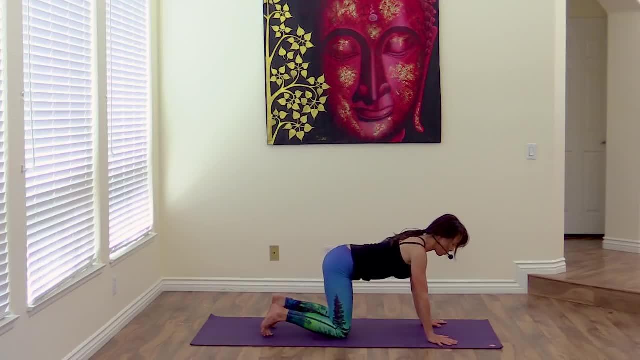 If your shoulders are tight, maybe a little bit wider, Okay, when I say turned out, I don't mean like this, Okay, so just slightly. Tuck the toes, lift the hips up, Make sure that the feet are parallel. 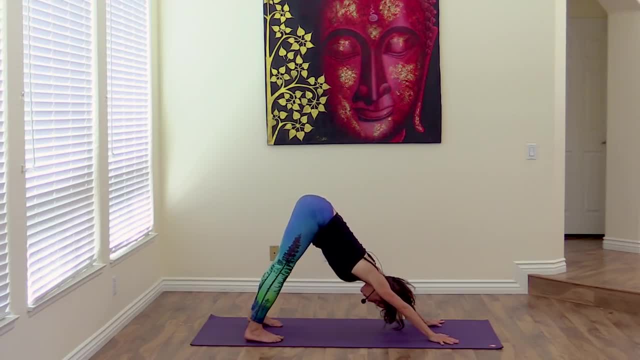 So you can even separate the feet a little wider if your hamstrings are tight, And then find a stretch in the upper back. Now your heels may be up really high. I've been doing yoga for 20 years, Every single day, So I'll tell you that my hamstrings are more open. 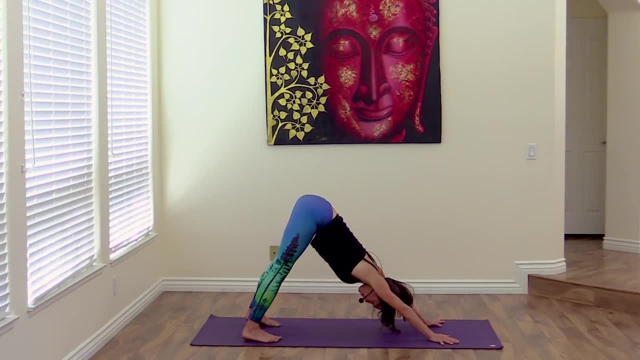 But when I started yoga they weren't And my upper body wasn't strong. In fact, I wasn't strong, flexible, coordinated or any of that. So it does take time, but it's well worth it. See if you can push up out of your shoulders. 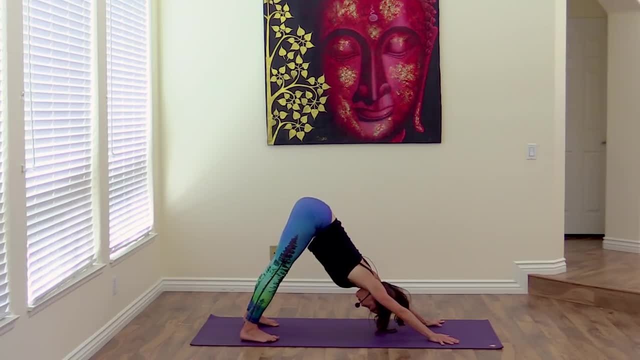 And take one more breath here, Good. And then set your knees down on your mat, Sit back on your heels- Child's pose. Rest your forehead down- Good. Okay, let's come up again. Hands and knees first. Tuck the toes. 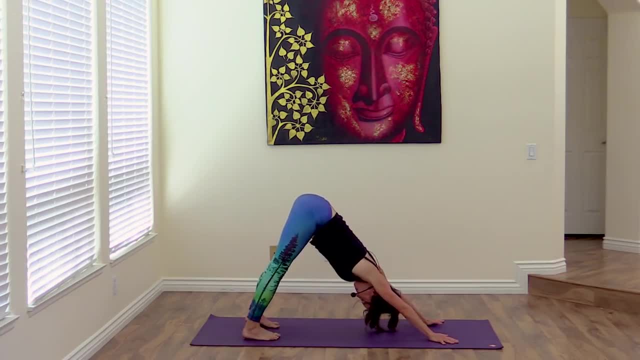 Push up and back to downward facing dog Feet. parallel Activate the upper back so that you feel a stretch big time. I know it's a lot of strength too. See if you can hug the belly in a little bit. Lengthen through your spine. 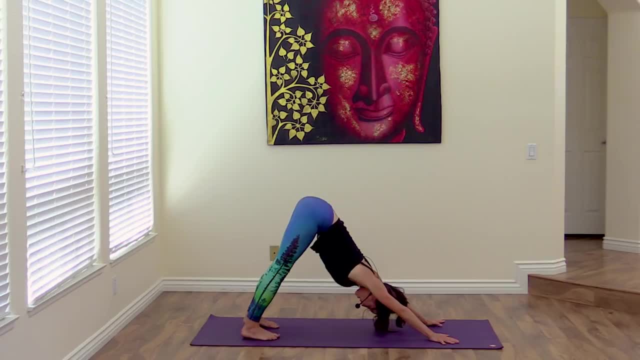 Breathe And then, knees back down, Sit back on your heels. I'm a proponent of moving in, not staying too long, but doing a couple sets. This is how you will build the stamina, as well as the strength and the range of motion. 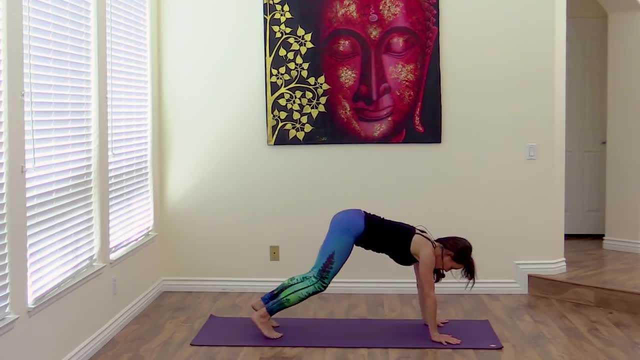 Okay, come on up one more time. Toes tuck, Hips lift, Push the floor away from you. Good, And then from here you'll step your right foot up to the front of your mat. You can scoot the right foot up with your hand if you need to. 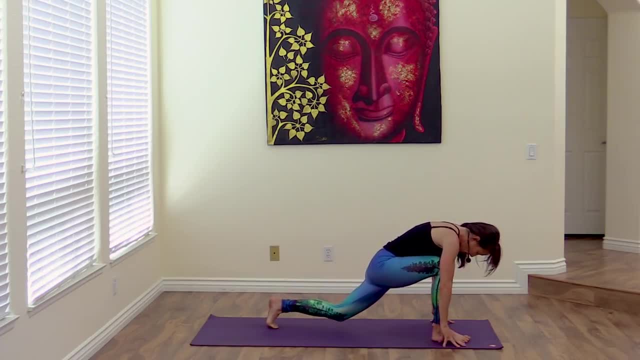 I know that that can be challenging at first, And then you'll lower your left knee to the mat. If your knees are at all sensitive, you can pad up your left knee by putting a blanket underneath it. Now walk your hands up onto your right thigh. 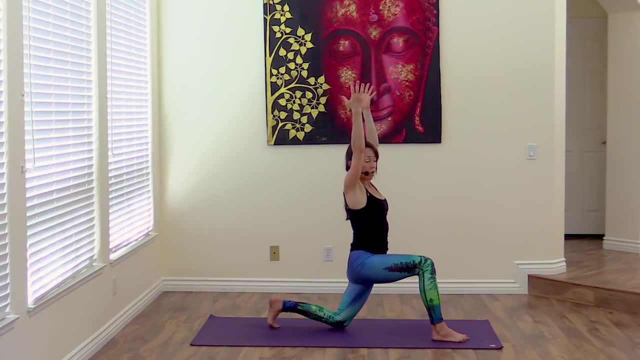 Reach the arms up, if you can. Now. if this is stress or strain on your shoulders, you can bend the elbows a little bit like goal posts. Otherwise, reach the arms up, Lift the belly in, Breathe Good And then release the hands down to the mat. 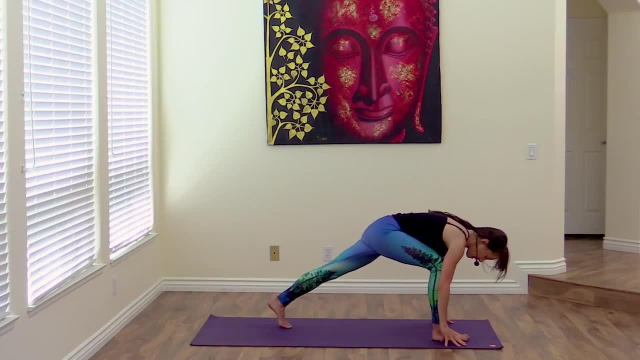 Tuck the back toes, if they're not already, and lift that left knee up. Lift the left knee up and be in a runner's lunge Now. just be mindful that you're not rounding in or hunching over. Get the length of the spine. 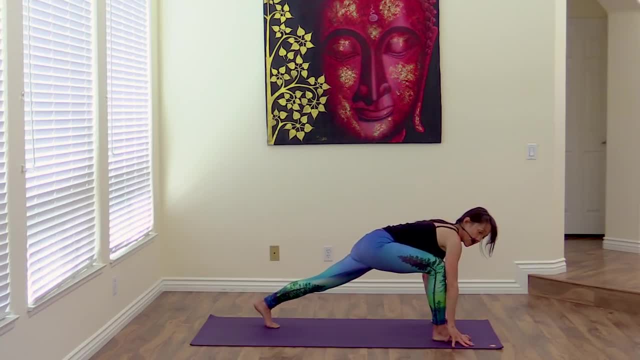 Feel the right hip, hug into center so you're not collapsing out to the side. Good, And then step the left foot up to meet the right foot at the front of your mat On an inhale. take your hands onto your shins gently. 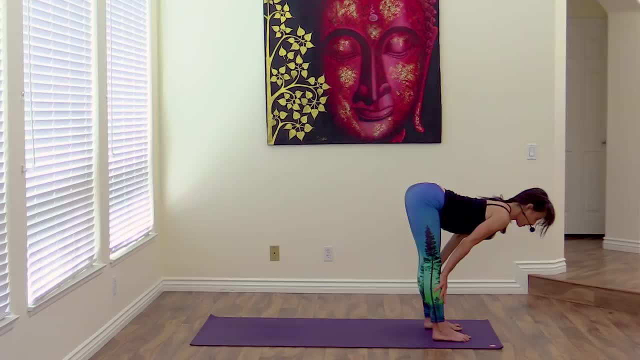 Lengthen the spine forward, Get the length And then fold forward to any degree. on the exhale- Good, On an inhale- you're going to come all the way up to stand. Firm the belly to support your spine, Reach the arms up. 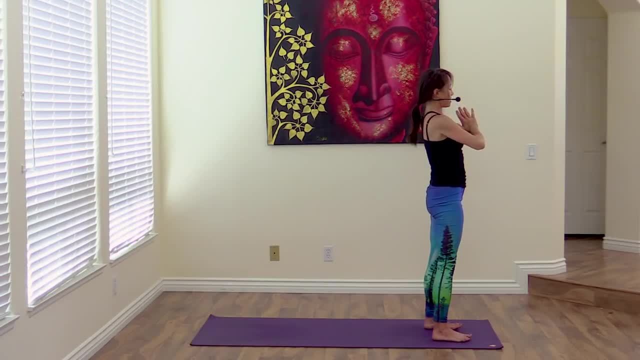 And palms connect in front of the heart on the exhale- Good Inhale. the arms reach up And exhale. fold forward On an inhale. hands come to the shins. Lengthen the spine so that you're almost at a 45-degree angle here. 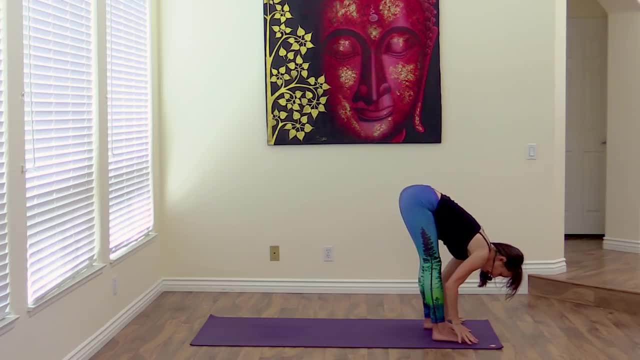 And then, as you exhale, plant the hands down to your mat, Step back to downward facing dog pose. Good, And then from here you'll set your knees back down on the mat, Shift your body weight a little forward and lower all the way down to the ground. 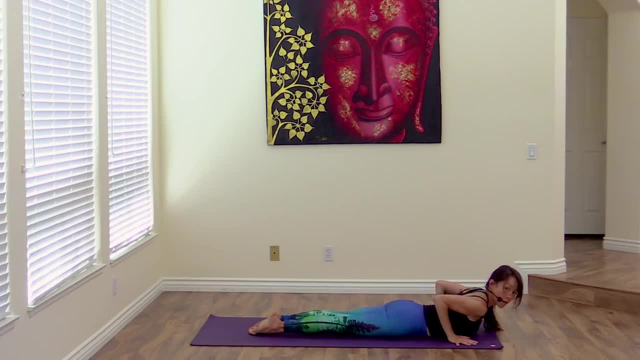 Good. Release your toes so that the tops of your feet are on your mat. Turn the heels out a little bit. Toes in The elbows hug in by the rib cage as we come up into cobra pose. So, on an inhale, press your chest up a little bit. 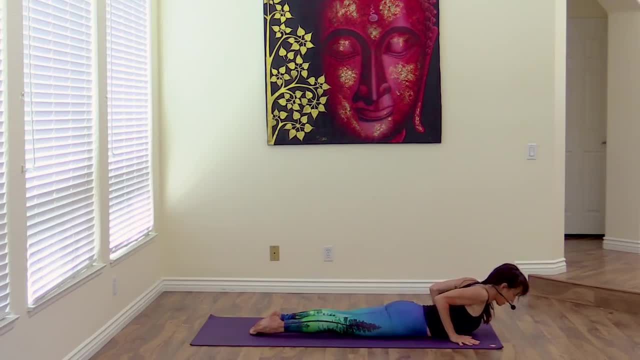 And then, as you exhale lower back down, Good Inhale. Press your chest up. Exhale lower down Doesn't have to be very high, It can be just a little bit. One more time Inhale. 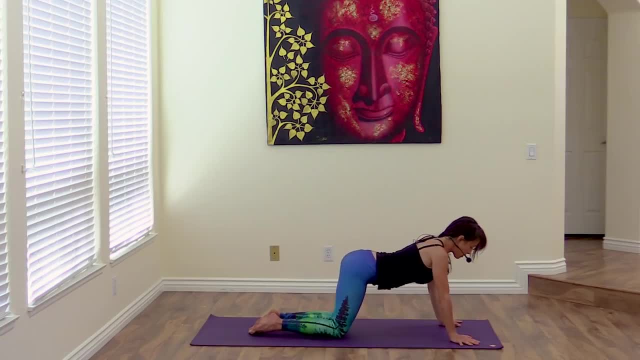 Press up And then exhale back to child's pose. Use your belly to assist you in your transitions. Good, Downward facing dog Deep breath, Good, And then you'll step your left foot up to the front of your mat. 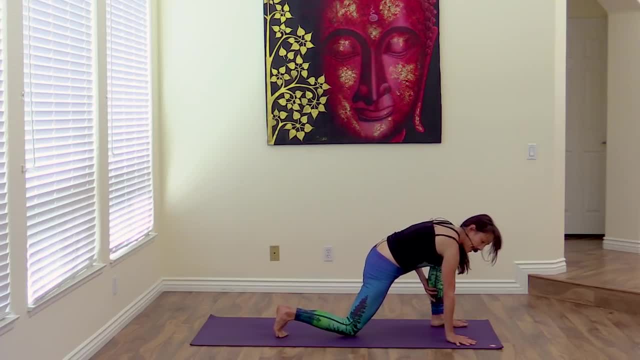 Assist the foot up if you need. Lower the right knee. Both hands climb up onto the left thigh for a moment. Good, Still breathing. Arms reach up. Be mindful that you've engaged your low abdominals So you want to lift the belly up out of your hip crease. 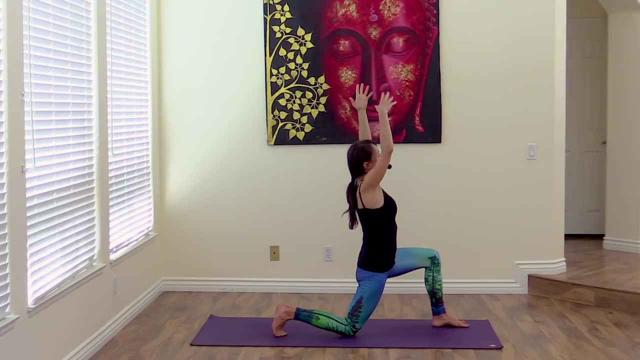 Shoulders soft. Soften your gaze So that your eyes are gentle, Breathe deeply. It's all about the breath. Smooth and steady, Good. And then hands down to the ground, Be on the fingertips. You can also take blocks, yoga blocks- under your hands. 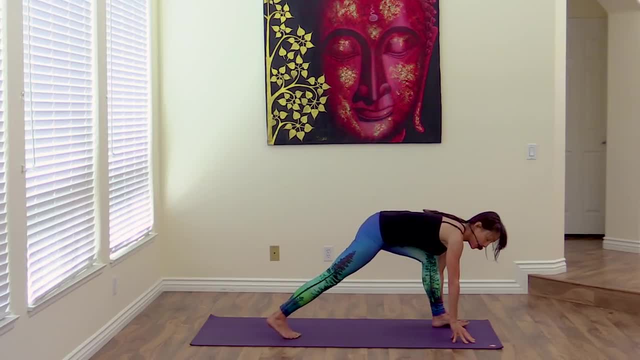 If you've never done yoga before, you probably don't have any, But if you do, you can use them. Tuck that Back toes, Lift that right knee And be in a runner's lunge here. So the left knee is at a 90 degree angle. 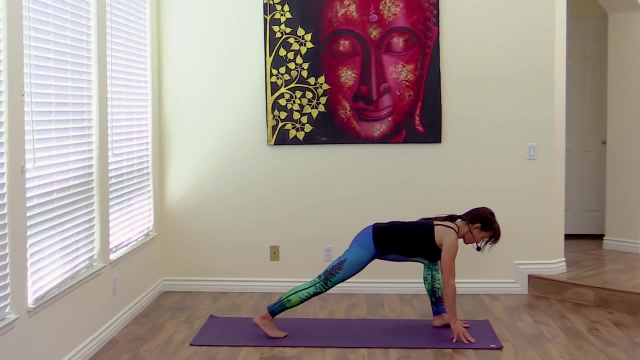 And the right leg is as straight as you can get. Lengthen your spine, including your neck. Shoulders slide away from the ears. Good. Step the right foot up to the front of your mat, Feet about hips width apart And parallel the feet. 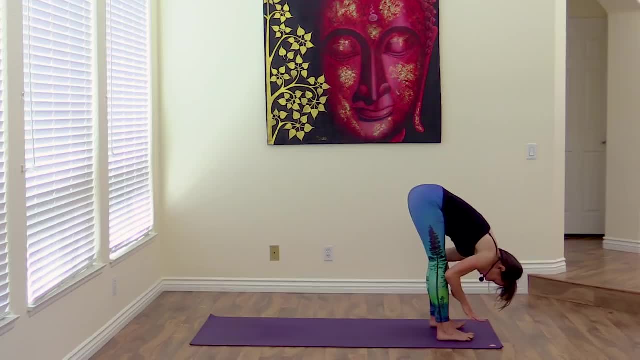 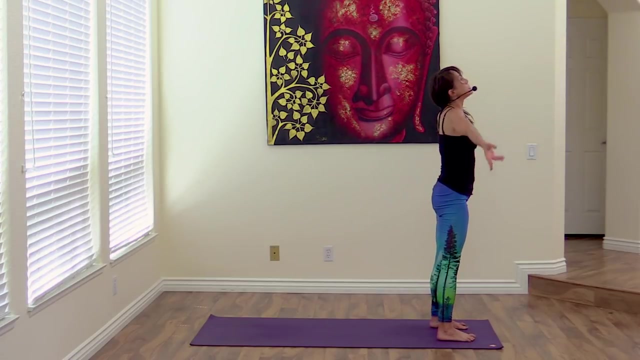 Be mindful that your toes don't turn out On an inhale, hands on shins. Lengthen the spine As you exhale. fold forward As you inhale, belly in Rise all the way up to stand up. And as you exhale, palms connect in front of the heart. 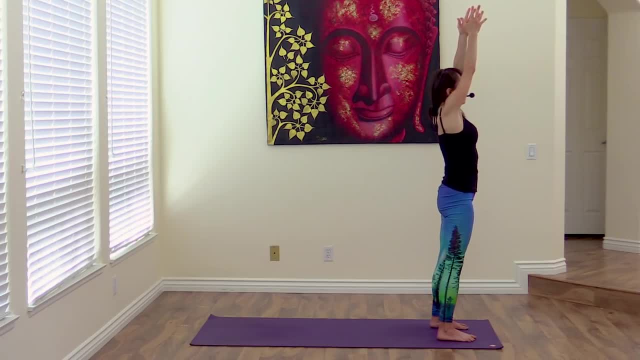 Inhale the arms, reach up, Exhale, fold forward, And we'll do that one more time. Inhale hands on shins, Lengthen As you exhale, fold in Good, Linking the breath and movement. 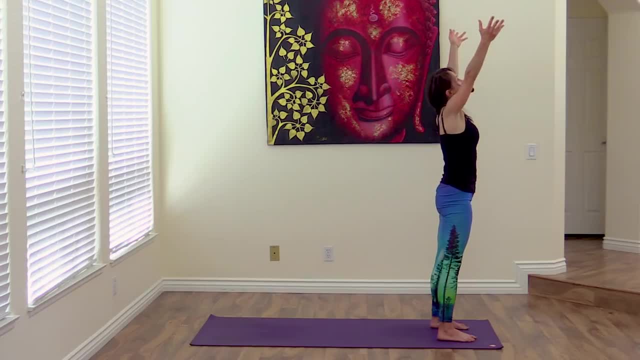 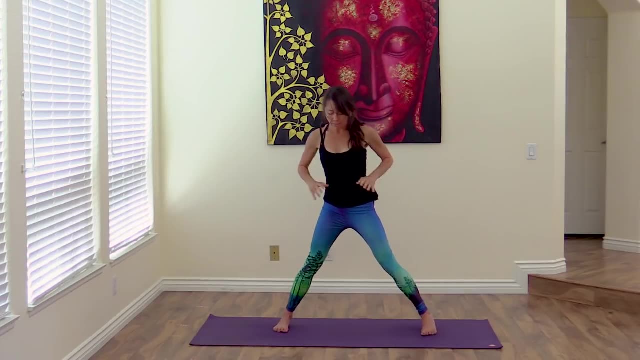 Inhale. Rise up to stand up And exhale the palms. meet at the heart. Good, Okay, From here we'll take a wide step on the mat, Wide enough that you can get your heels A bit wider than your shoulders. 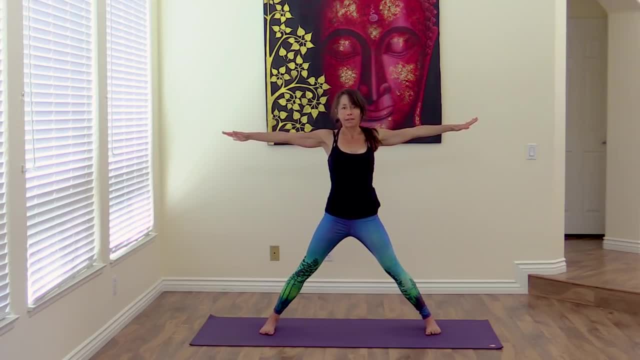 When you take your arms out, ideally so that the wrists and the heels are about aligned Approximately. Okay, From here you'll turn your right foot out So that it aligns with the right edge of your yoga mat, So we don't want the toes turned in or turned out. 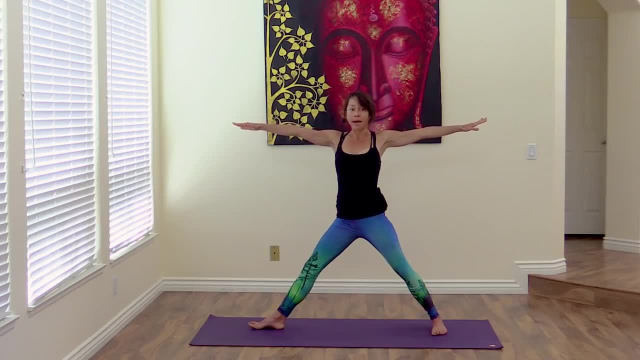 We want the right foot to be straight Arms up. Bend your right knee. This one's called Warrior Two Pose. Bend the right knee and be mindful that the right knee tracks over the right middle toe, So it's not collapsing in, It's not opening too wide. 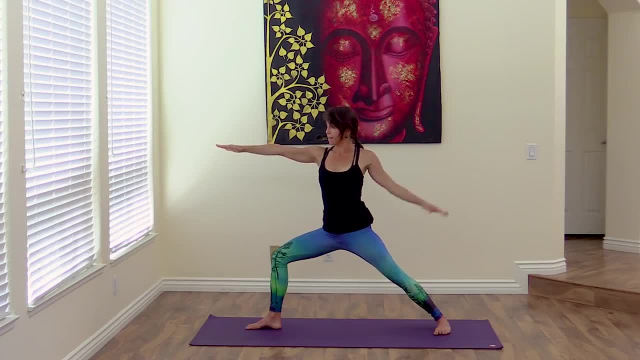 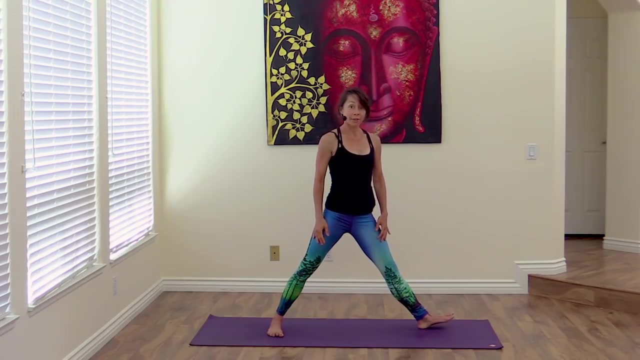 Right. Take a couple of breaths here. Back leg, left leg straight. Soften your shoulders, Deep breath. Good. Stretch the right leg straight. Release the arms down. Turn the right foot in, Left foot turns out Same thing. 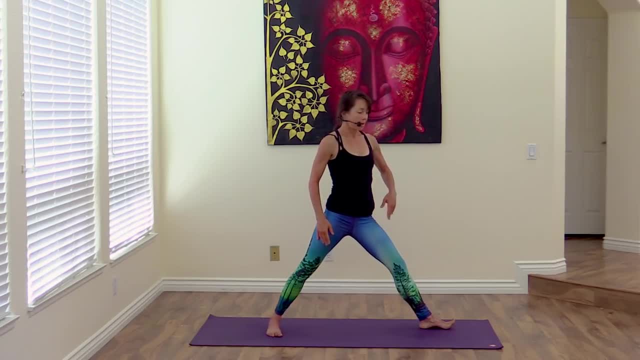 Align your foot with the left edge of your yoga mat. Bend the left knee. Left knee aligns with the left middle toe Warrior. Two Pose Deep breath, Shoulders soft- You can put a little kindness in your eyes, Beautiful. And then left leg straight. 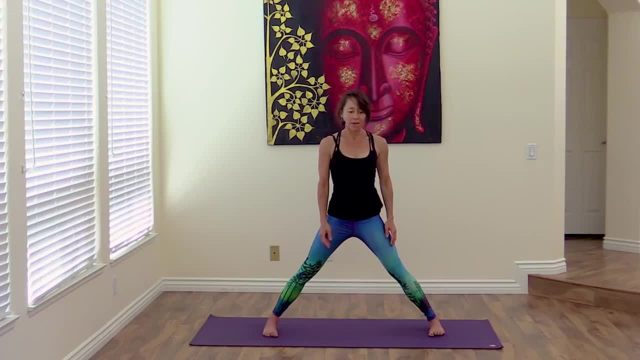 Lower the arms. Parallel the feet. Good, Let's bring the feet together for a moment. Shake out your legs- Okay, and then we'll separate the legs again. Same setup with the legs, Same width. Turn the right foot out. 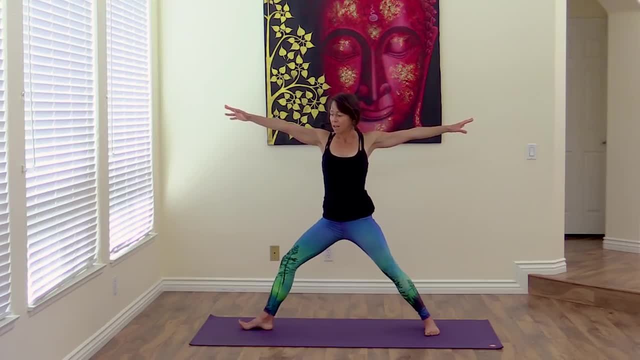 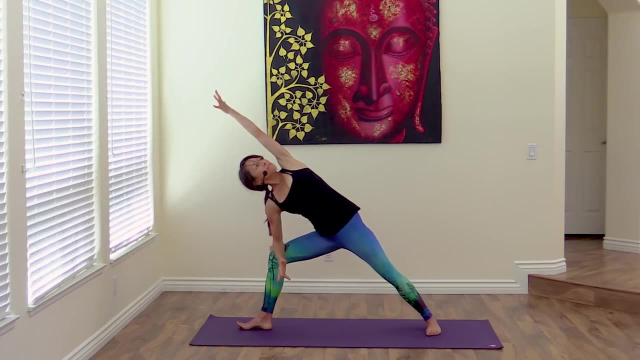 Arms out to your sides. Bend the right knee, This time right elbow to the right thigh. Left arm. reach over the left ear for a side stretch. This is called Side Angle Pose. Take a couple of deep breaths, Feel the right hip, hug in so you're not sticking your butt out behind you. 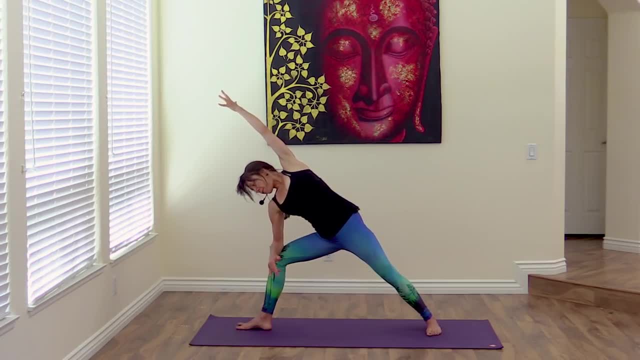 Hug the right hip in and be mindful that that right knee and the right middle toe are pointing in And the right middle toe are pointed straight forward to the front edge of your mat. One more breath, Good, Come up. Turn the right foot in. 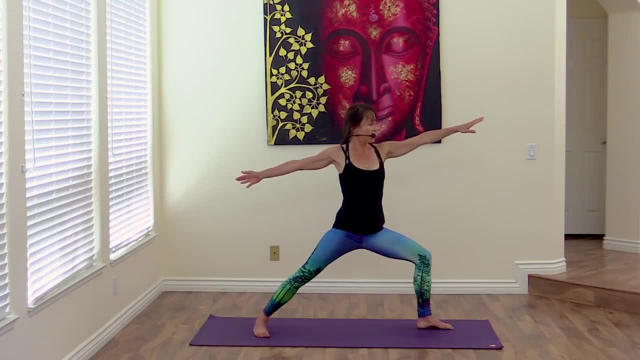 Left foot turns out. Bend the left knee. So we start from Warrior Two: Left elbow to the left thigh, Right arm, reach over the right ear. This is a dynamic pose. Lots of side stretch here. Make sure that right leg is engaged firmly. 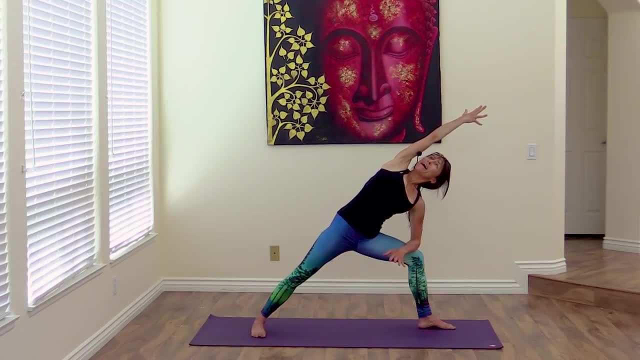 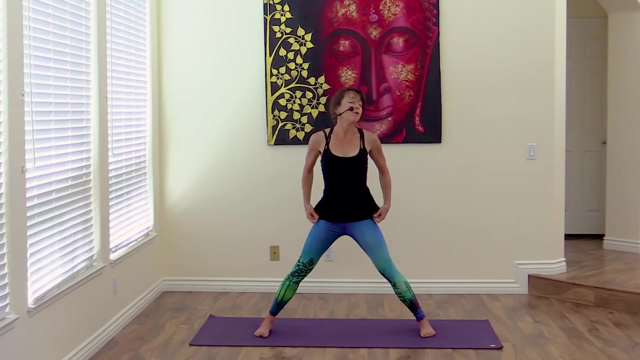 Shoulders slide down the back so you have space around your neck. Breathe Good And then come up Parallel the feet. Okay, from here we're going to take a standing forward bend, which for some of you will be easy. 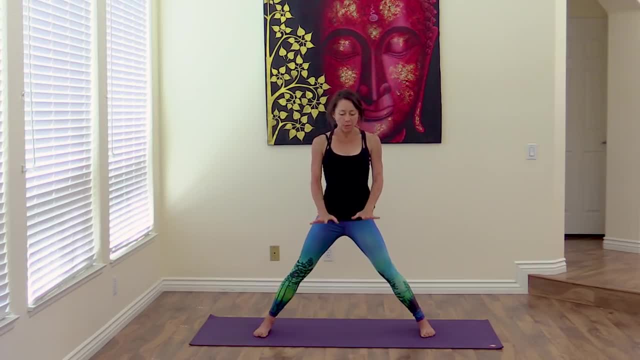 and some of you, it might be a lot more challenging. You can take something to prop your hands up. This is where yoga blocks can come in really handy. You can pick them up online for probably $10 each. They're not expensive. There's loads of places to get them and you don't need anything special. 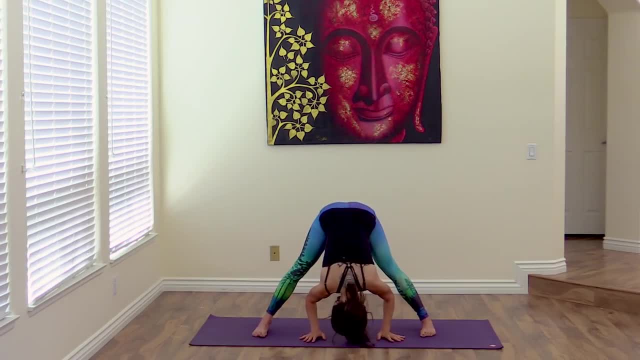 Fold forward And then from here in your forward fold. if you've got your hands on blocks because you can't reach the floor, that's fine. If you do reach the floor- which is actually pretty rare in beginners- then great, grab the floor. 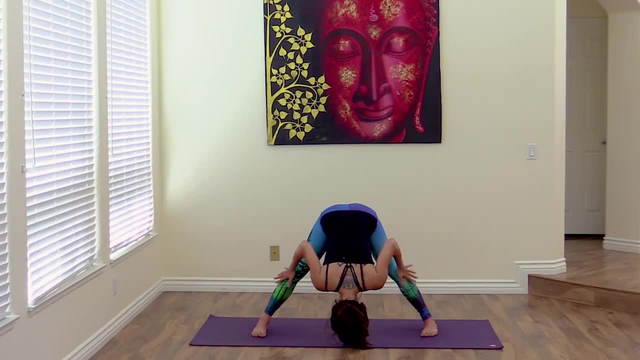 But grab something You could also grab onto your legs, but just be sure that you're not putting any pressure or any weight on your kneecap. if you do that, Relax your neck. Relax your neck and deepen your breath. Good, Come on up. 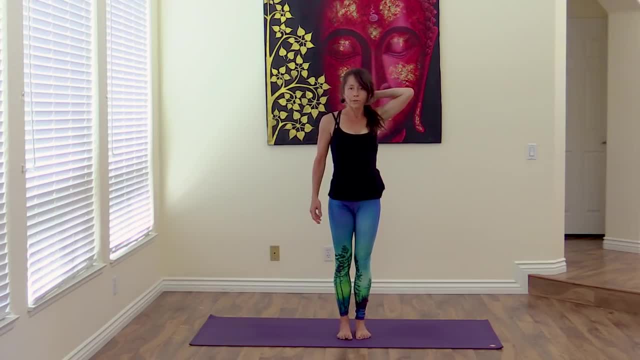 Bring the feet together And we'll do one last bit of standing balance before we hit the floor again. This one's called tree pose. You stand on your right leg, okay? One of the keys to balance, by the way, is to look at something A that's not moving. 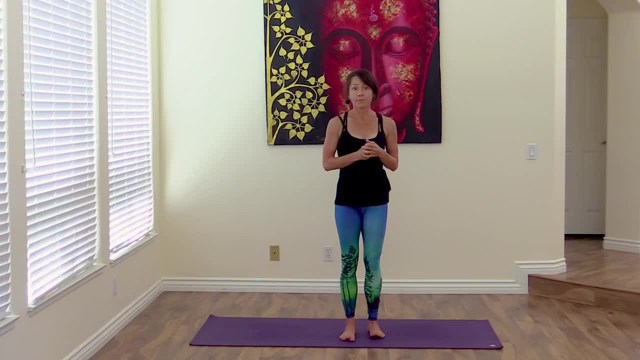 and B, ideally something that's kind of close to you. Another suggestion is: try not to look at a white wall. It's very hard. It's still almost impossible for me to balance staring at a white wall. You can start with your left toes on the floor. 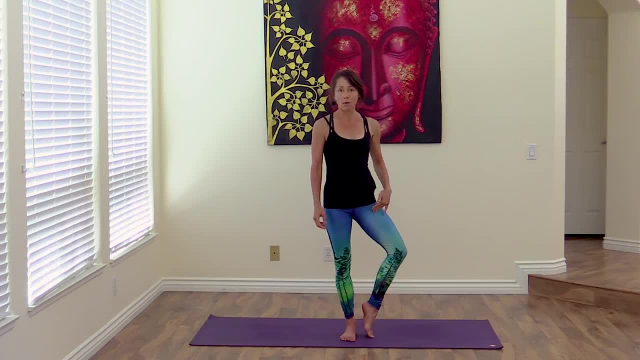 The left knee will rotate outward. It's really not even the knee, It's the whole left hip, the whole left leg. So you can start here and bring your palms together in front of your heart And, if you want to add more, 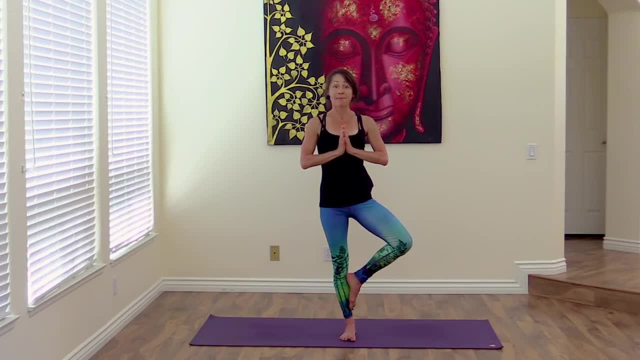 you can maybe take that left foot up to the right thigh and play with that for balance, And if you've got the range of motion and your balance feels pretty steady, you can take that left foot up to the right thigh. Again, no pressure on that knee joint, please. 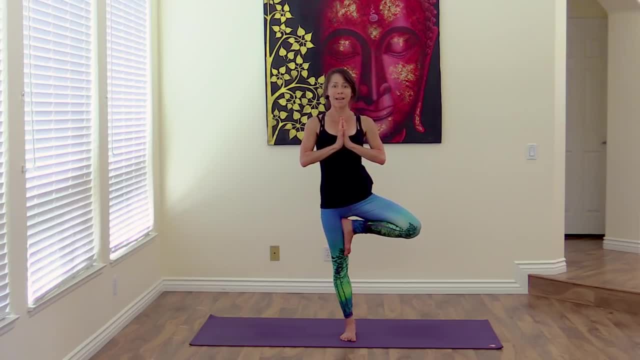 on the right knee, joint Palms together in front of your heart, A couple of very deep breaths. Be prepared to wobble a little bit or even fall. If you fall, you just get back in. If you wobble, this is part of just being human and falling. 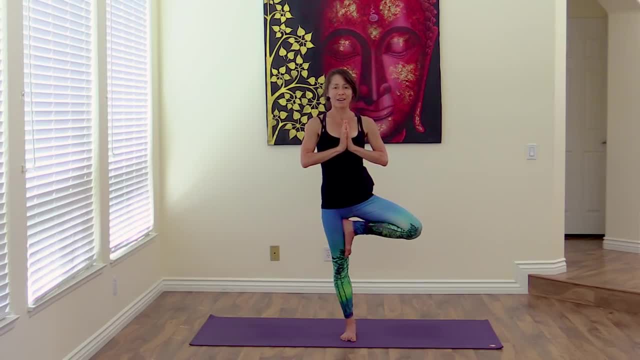 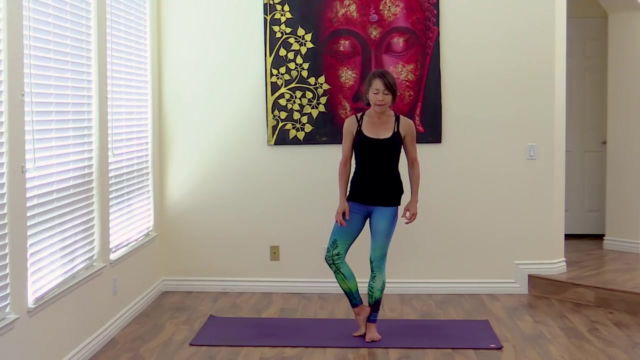 Everyone falls, Not everyone gets back up. So get yourself back up, Try again And then release And we'll switch sides So you can start with the toes on the floor, if that's helpful to you, And then eventually you'll take that right foot up to the left calf. 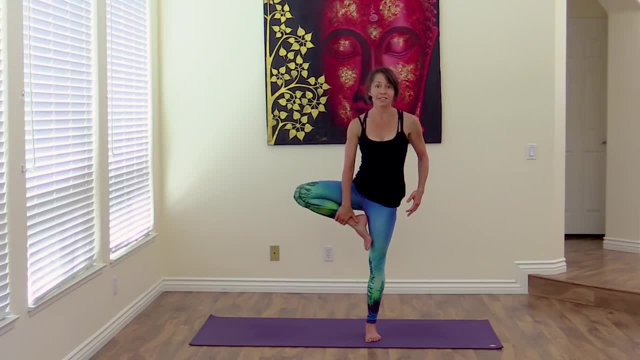 And then maybe, if it feels good to you, you can take the right foot up onto the left, thigh Palms together in front of your heart. Just FYI, it's not supposed to be a certain way. Okay, It never is. 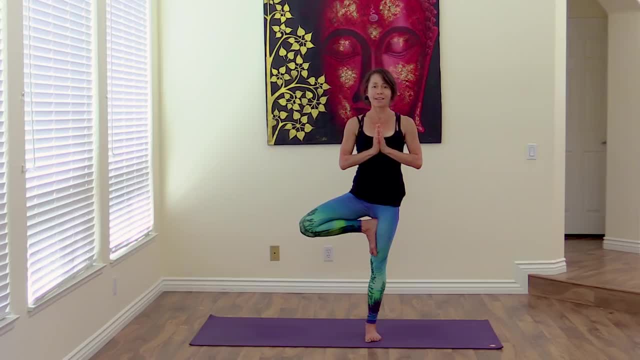 Aside from the way that fits your body. Okay, so let's just say that The specific way that it's supposed to be is the way that fits your body perfectly, The way that allows you to breathe most deeply, Relax your jaw, Relax your gaze. 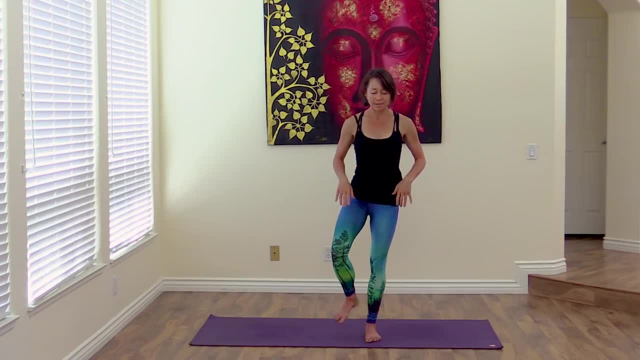 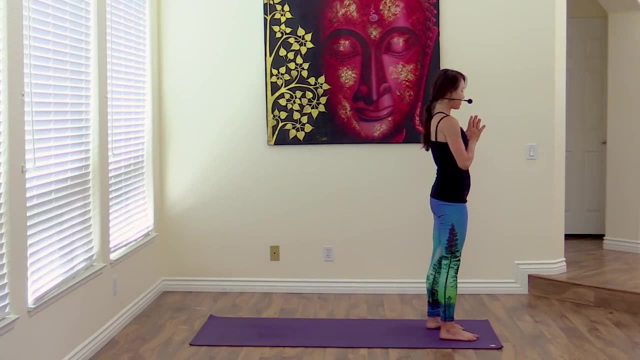 Good And then release. We'll come back to the front of the mat. Feet, parallel Palms together. Inhale The arms up. Exhale Fold forward. Inhale Hands on shins. Lengthen the spine. 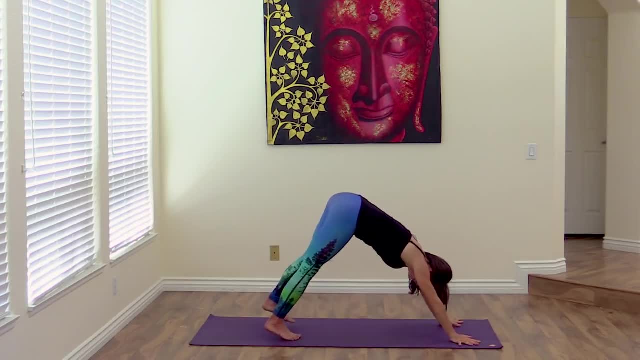 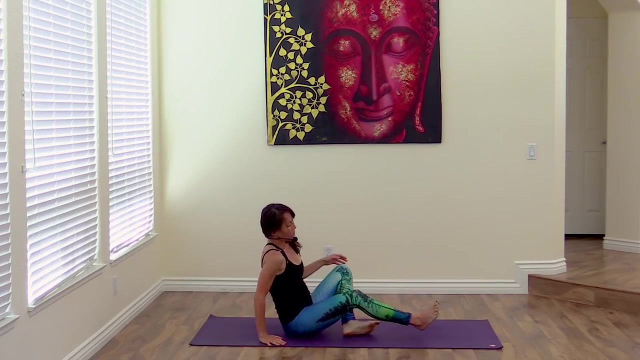 And exhale. Step back one last time Downward, facing dog pose. Good, And then from here you'll set your knees down on your mat, Cross your ankles behind you, Sit back onto your bottom, Stretch the right leg straight in front of you. 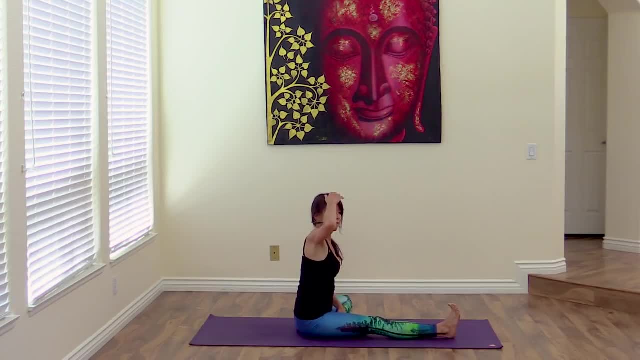 Left knee bends out to the sides. Now, if your hamstrings are on the tighter side, you might want something to put around your right foot like a strap. a yoga strap or a towel works fine. You can also grab your right leg. 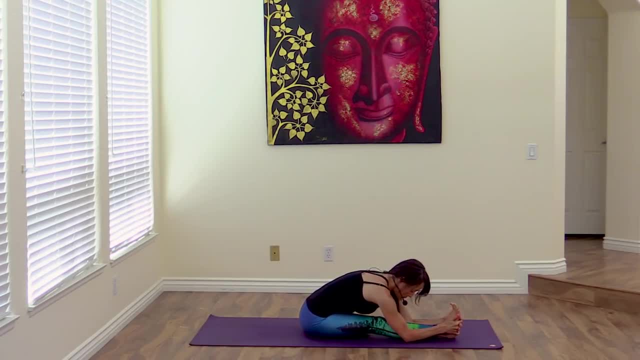 If you can easily grab your right foot, you can do that: Relax your head, Deepen your breath, Get space around your neck. Good, Okay, Come on up. We're doing intentionally shorter holds: Left leg straight, Right knee bends out to the side. 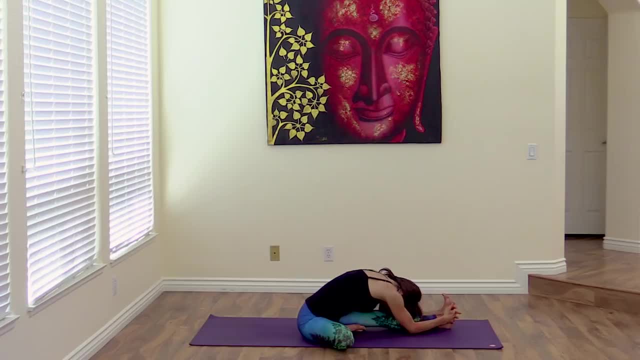 Fold forward, Grab what you can grab. Left side and right side are pretty much always going to be completely different. That's okay. We're here to be present with ourselves, present in our bodies, Breathing. Relax your neck Good. 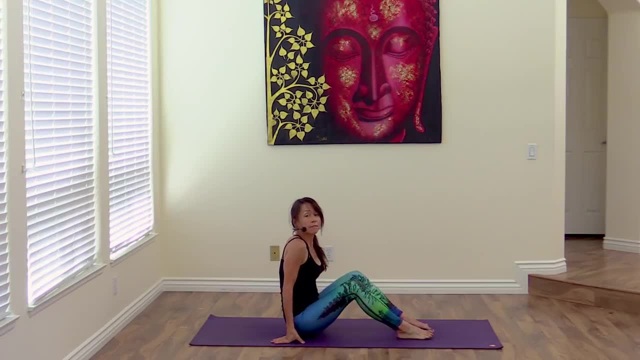 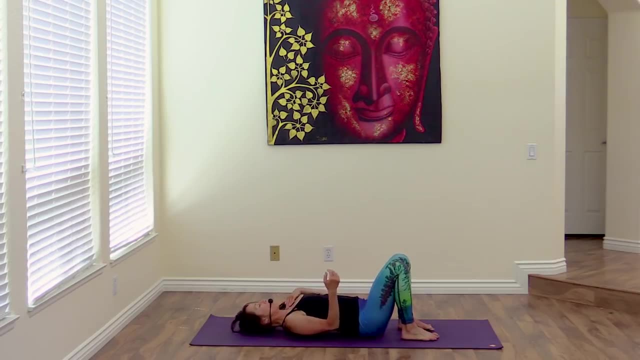 And then come on up And from here you'll bend your knees, feet on the floor, Lie all the way down onto your back. please Lie down onto your back And just take a moment here and notice how you feel. We want the feet just close enough to your hips. 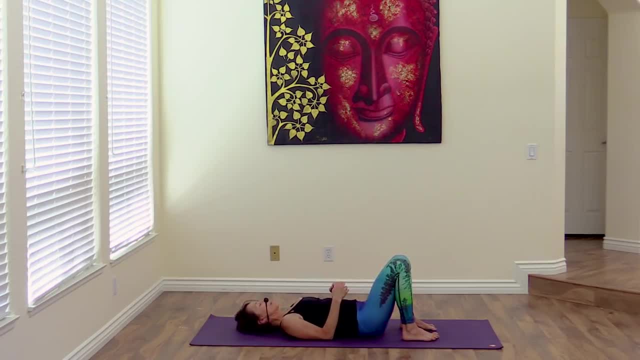 so you can touch them with your hands. Okay, And then from here, we'll bend the elbows with the fingertips pointing upward. So, point your fingertips upward. Elbows, bent Elbows on the floor. From here you'll roll the hips up. 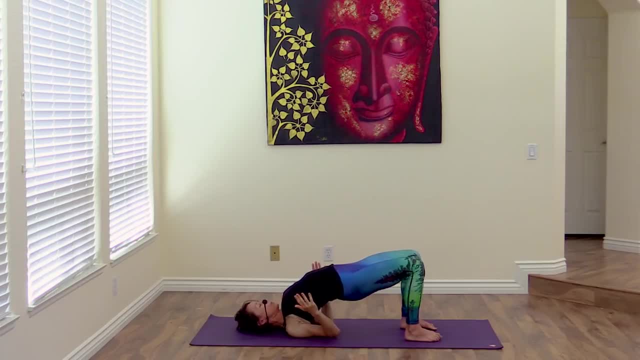 Roll the spine up off the floor, Walk the shoulder blades together under your back And continue to press elbows and upper arms down, heart up. The feet press down, especially the inner edges, the big toe side of your foot, Press it down. 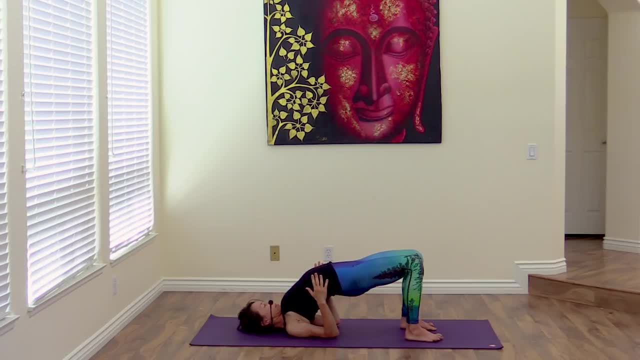 Lift the chest up more Breathing Good, And then unroll the shoulders, Come back down onto your back. Take a moment to notice how you feel Beautiful Now. right ankle, cross over the left thigh. One more stretch. here you guys. 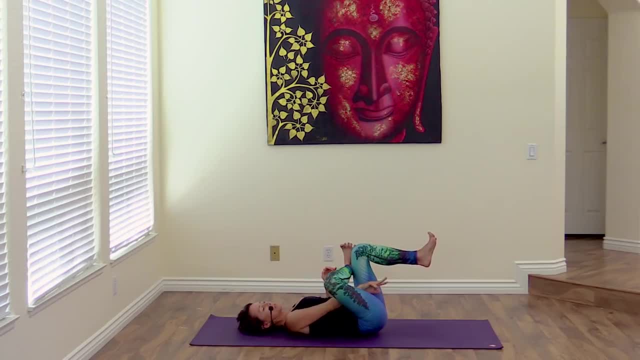 Lift the left foot up off the floor. Right hand goes through this triangle between your legs And you grab the outside of your left leg, your hamstrings on your left leg, with your right hand and also, with your left hand, Flex the feet, both of them, to protect your knee joints. 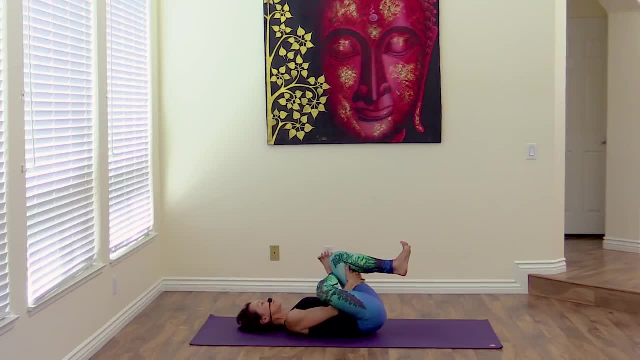 And gently draw your legs in toward you, even if it doesn't feel like it's very far. The idea is to get a good stretch in your right piriformis muscle, which is in the right hip, If you have a challenging time getting your head to the floor. 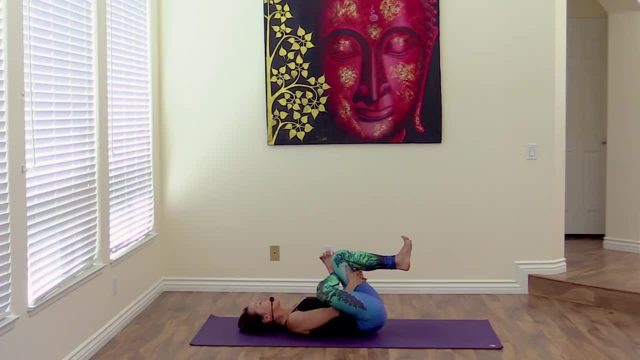 without straining your neck a lot or the upper back. then take a pillow or a yoga block or something under your head for support, to support your neck. Deep breath Through your nose right, Good, And then you'll release and switch sides. 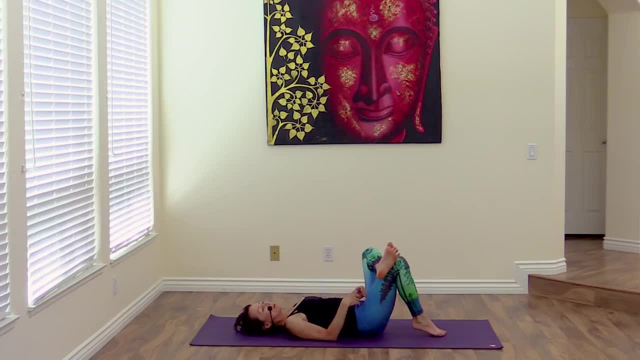 Left ankle cross over the right thigh. Lift the legs up. Grab the outside of your right hamstring with your right hand. The left hand goes through this triangle between your legs. Flex the feet And feel the shoulders sink down toward the ground. Breathe deeply. 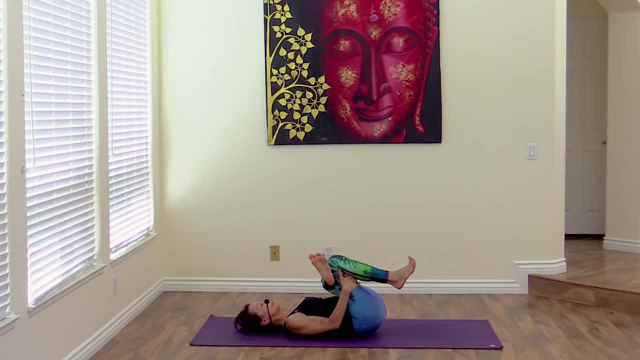 And see if you can slow the breath down. Smooth out the breath, Good, All right Release here. Stretch the arms and the legs straight to the floor. The final resting pose in yoga is essential to the practice. It's called Savasana. 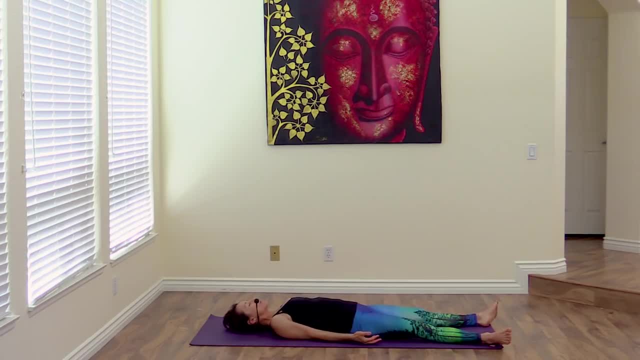 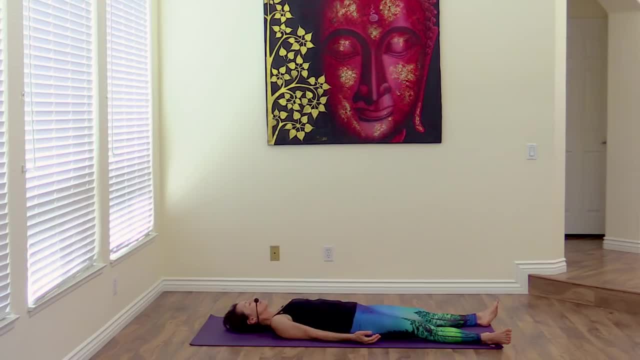 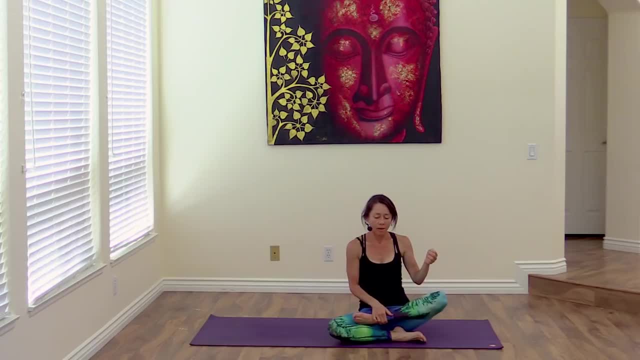 up to sit. sit however feels comfortable to you. allow your eyes to close for a moment, if that feels okay. do a scan of your body using your mind and notice how you feel good, and then bring your palms together in front of your heart and take a moment to acknowledge.